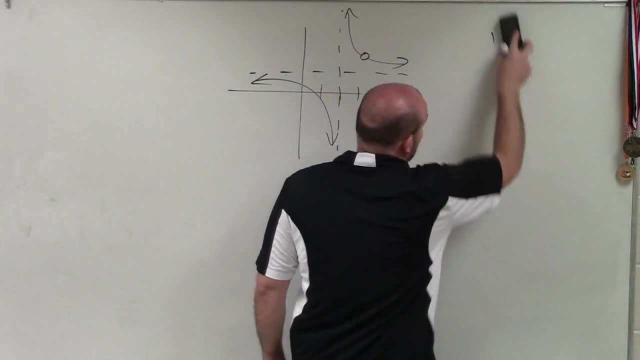 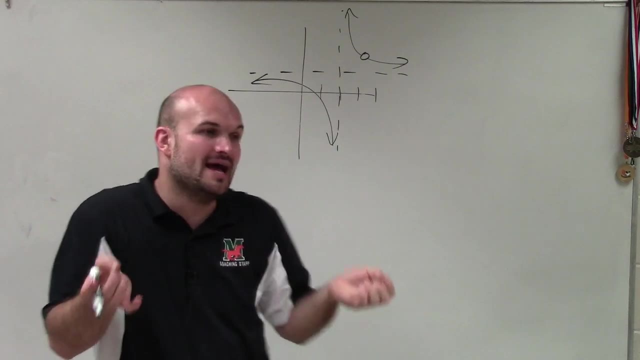 a graph of a rational equation or a rational function. what I want you to understand is: these dotted lines are what we call asymptotes, And that means our graph is not going to be a value at those lines. So here you can say that x cannot equal 2. And this value is an. 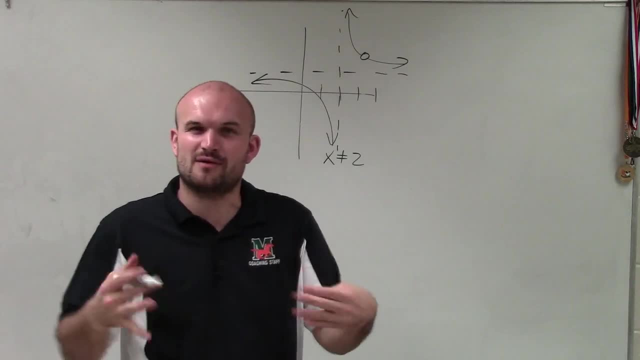 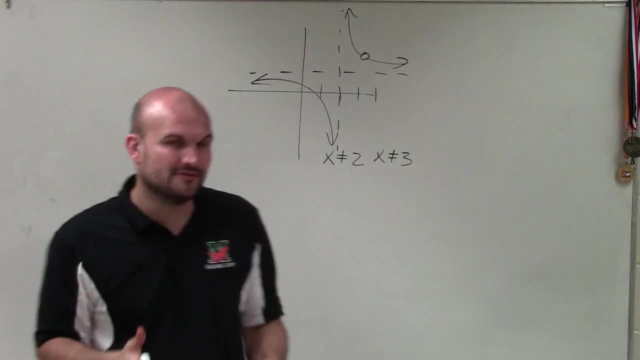 asymptote, And this is where the graph is going to approach, And I you know, I have other videos on what exactly asymptotes are- And then you could also see that x cannot equal 3, because that's a hole, And there's a difference between holes and asymptotes. 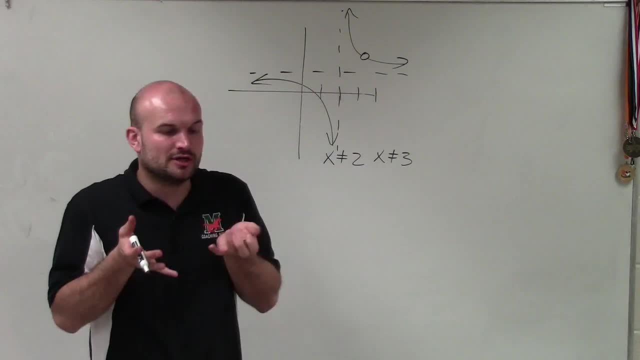 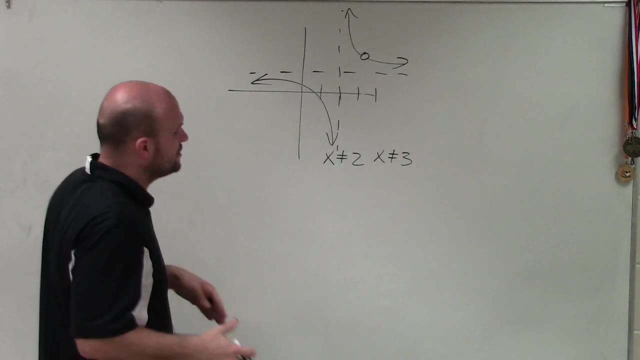 but their similarities are that both of them- your values- are not. they're not solutions of your equation. So let's go and look at well, how do these even come about as an equation? Because I can kind of see all right in a graph wherever there's that dotted line or there's an open. 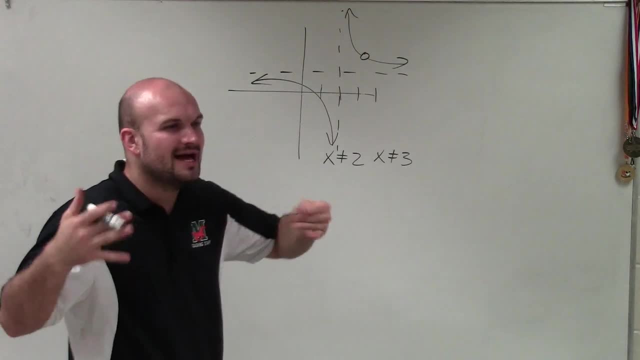 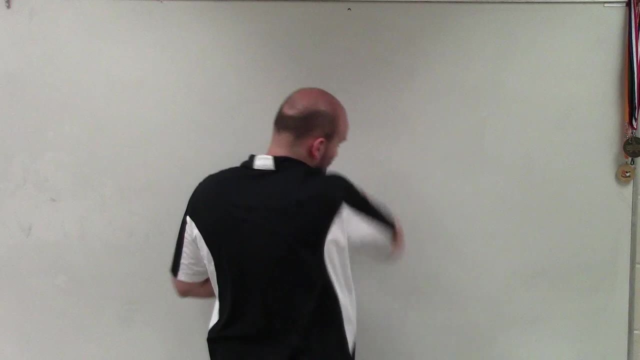 circle. that's a hole. They're not a part of the solution. Okay, I kind of get it, But how do we identify that in an equation and how do we solve, find them? So we spend a lot of time when graphing is finding the holes and finding the asymptotes. 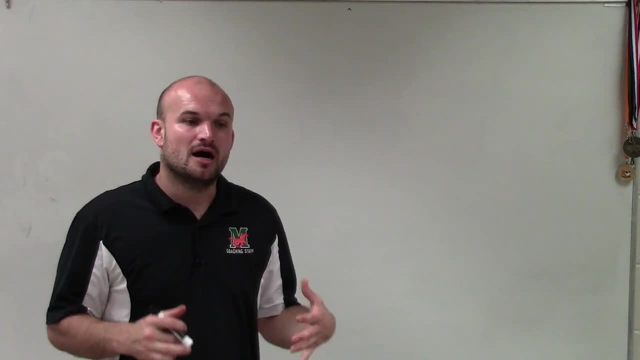 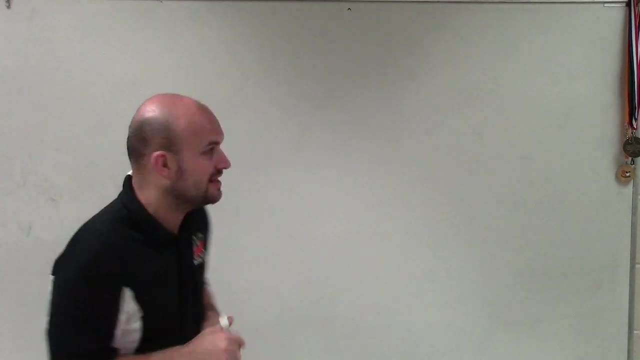 But you have to have a general understanding when we're solving rational equations because sometimes, even though we find a solution, our solution could be what the asymptote is or the hole. So we got to make sure we know how to identify them. And the best way to know how to identify 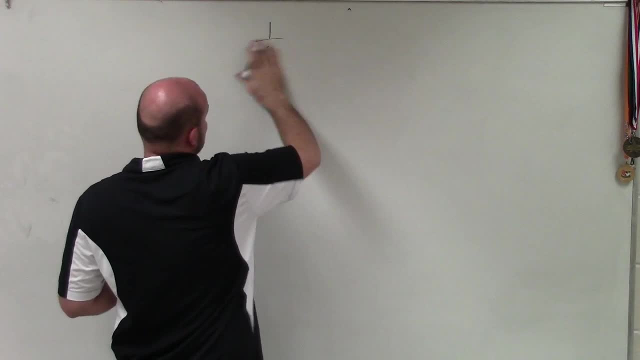 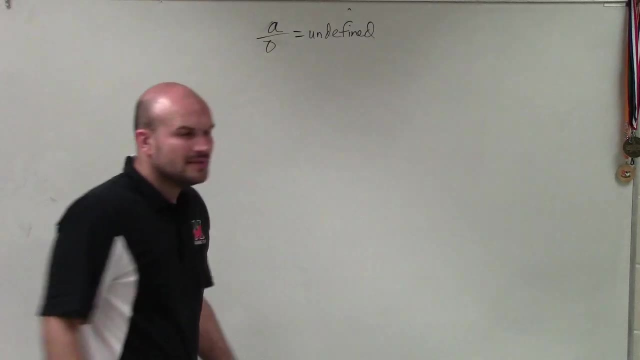 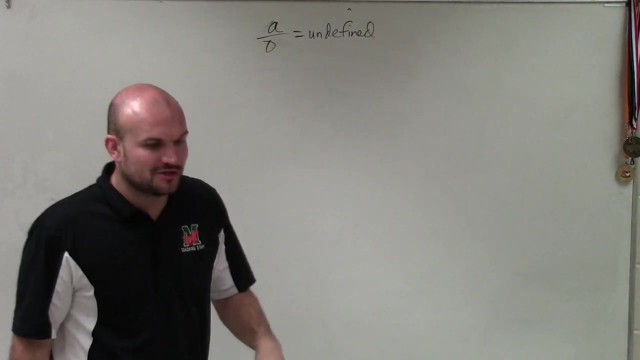 them is with a basic understanding that- sorry, a divided by 0 is undefined, Right, Anything divided by 0 is going to be undefined. You can't divide 0 into any number, no matter what the number is. So if we have this basic understanding when we're looking at a rational equation, 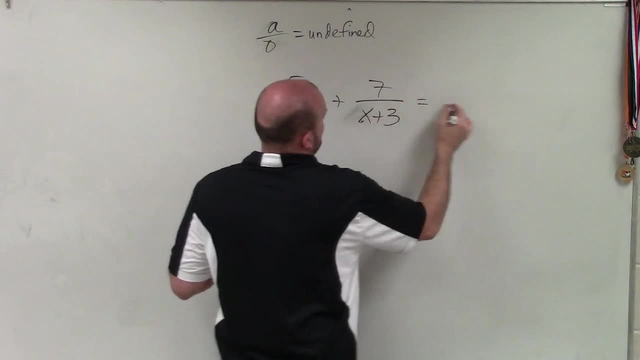 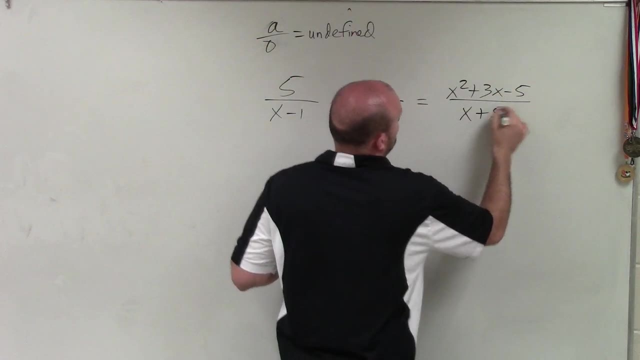 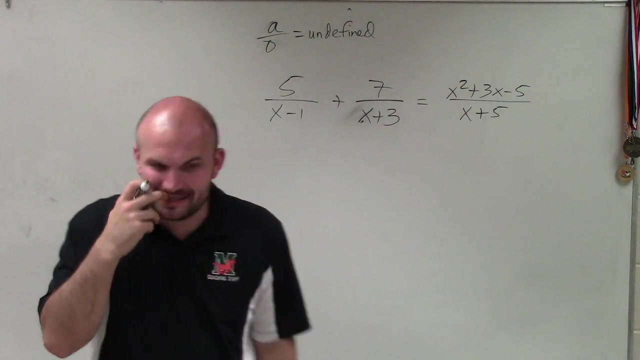 what we want to do when we're looking at a rational equation, even a crazy one like this I just made it up. But if we're looking at this, what we need to understand is all right. well, what I'm going to do is I'm going to put restrictions on my domain. restrictions. 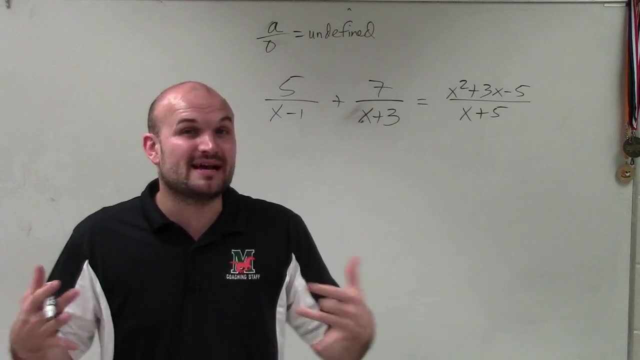 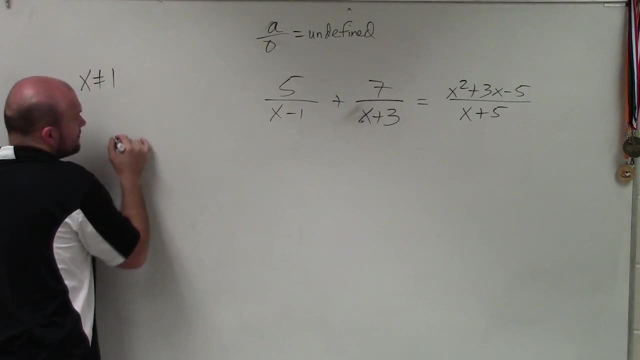 on my solution saying this: I don't know what the answers are, but I know when I get the answers. the answers cannot be these values, And the values that I'm going to choose are x cannot equal 1,, x cannot equal 3, or negative. 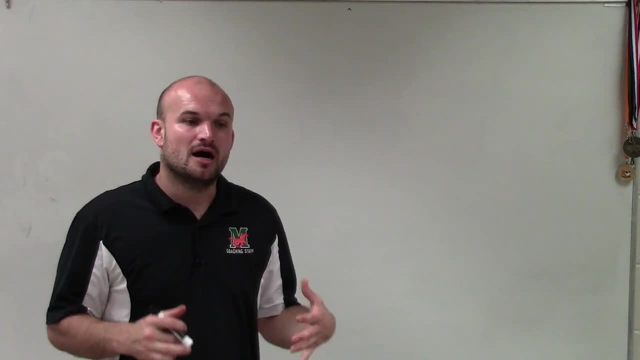 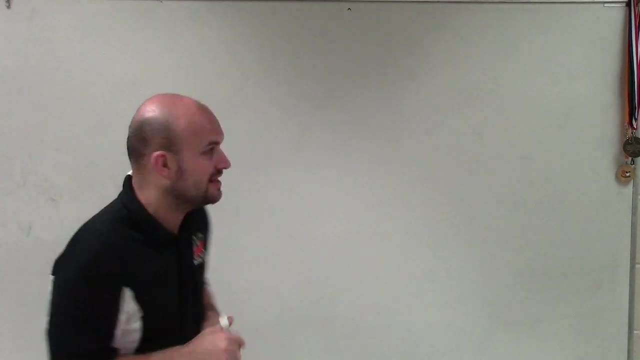 But you have to have a general understanding when we're solving rational equations because sometimes, even though we find a solution, our solution could be what the asymptote is or the hole. So we got to make sure we know how to identify them. And the best way to know how to identify 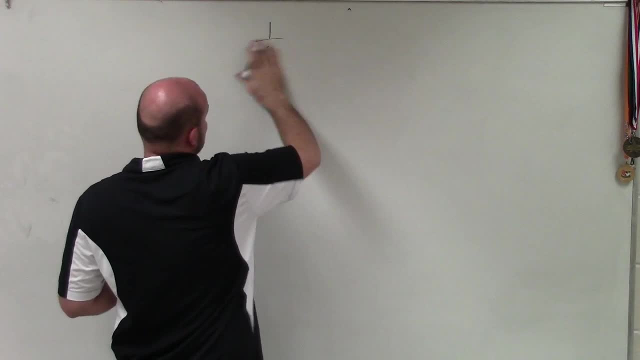 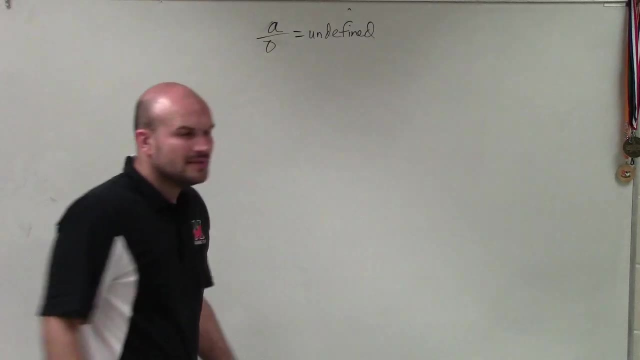 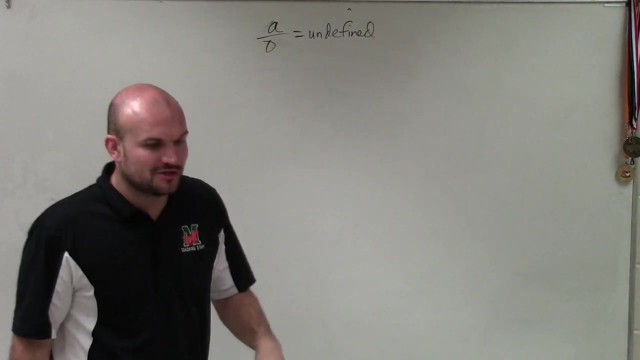 them is with a basic understanding that- sorry, a divided by 0 is undefined, Right, Anything divided by 0 is going to be undefined. You can't divide 0 into any number, no matter what the number is. So if we have this basic understanding when we're looking at a rational equation, 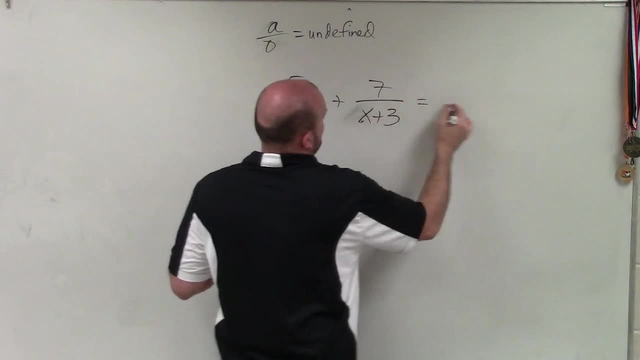 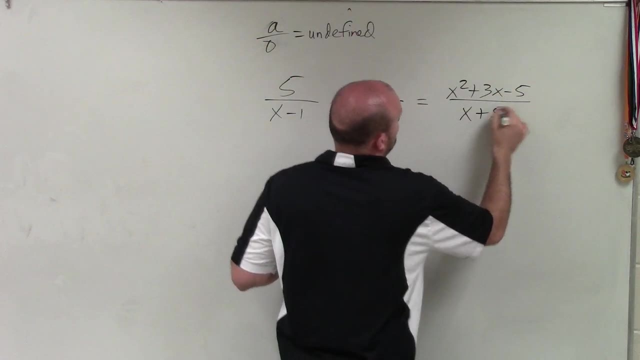 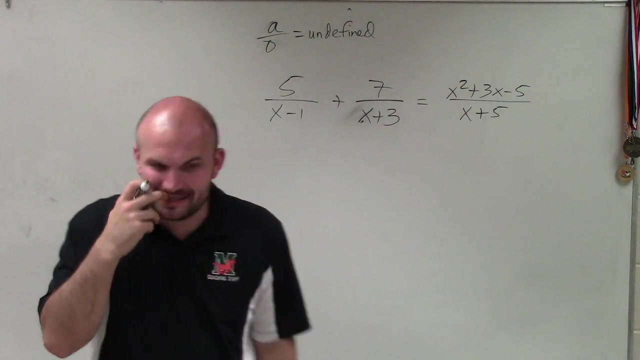 what we want to do when we're looking at a rational equation, even a crazy one like this I just made it up. But if we're looking at this, what we need to understand is all right. well, what I'm going to do is I'm going to put restrictions on my domain. restrictions. 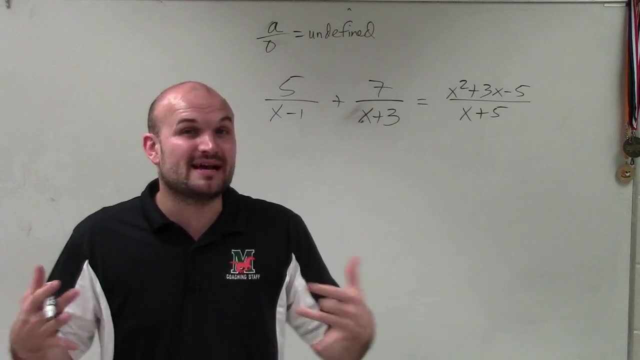 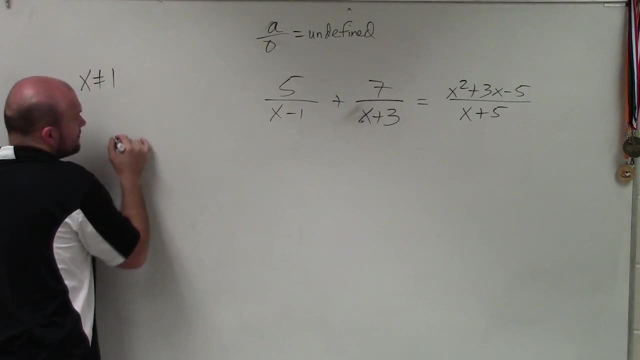 on my solution saying this: I don't know what the answers are, but I know when I get the answers. the answers cannot be these values, And the values that I'm going to choose are x cannot equal 1,, x cannot equal 3, or negative. 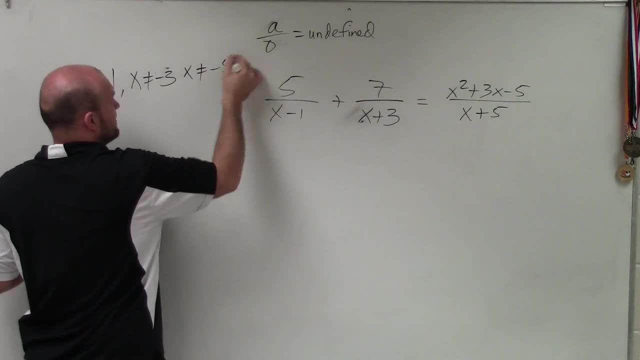 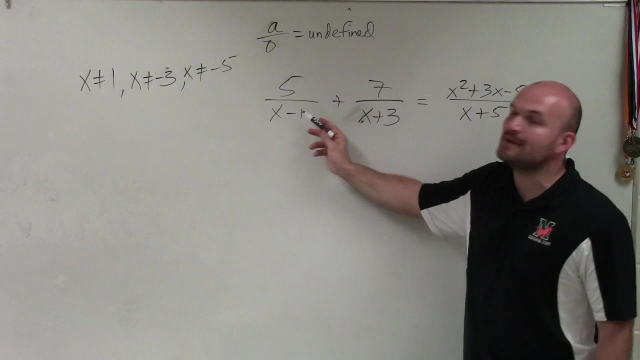 3, and x cannot equal negative 5.. Now, why am I choosing these values? Well, if I take 1 and I plug it in for x, you can see that 1 minus 1 is going to be 0. Therefore that 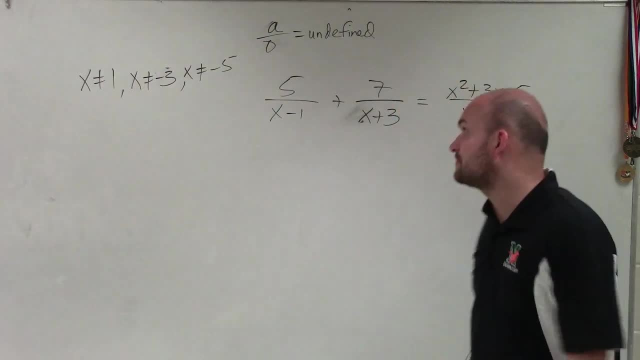 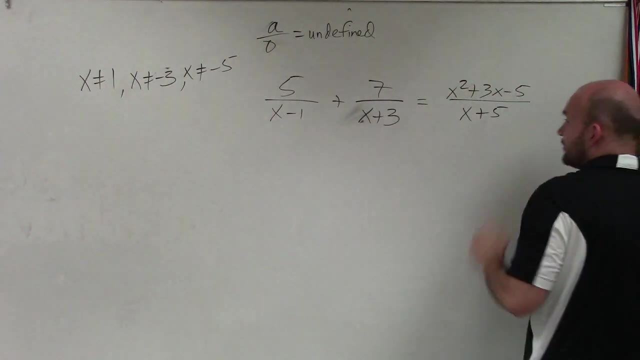 is going to produce an undefined value, which we call an extraneous solution. If I plug negative 3 in for x- you can see here- it's going to create 0. And if I plug negative 5 in for x over here, it creates 0. So any time we have a value that can create 0 in 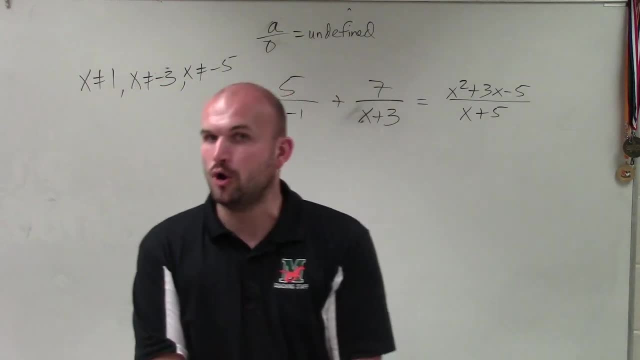 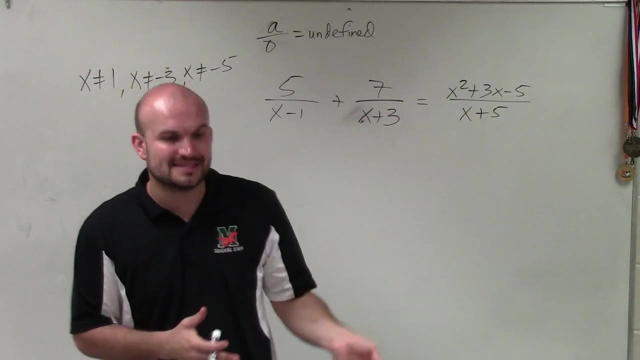 our solution. it is either going to create an asymptote or a hole, and the solution is going to be extraneous. Now the difference I'll go through real quick as far as a hole and an asymptote. Hole and asymptotes are very similar, but the difference between a hole and an asymptote is we can. 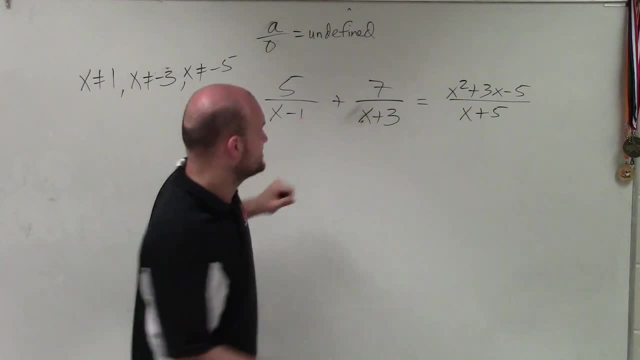 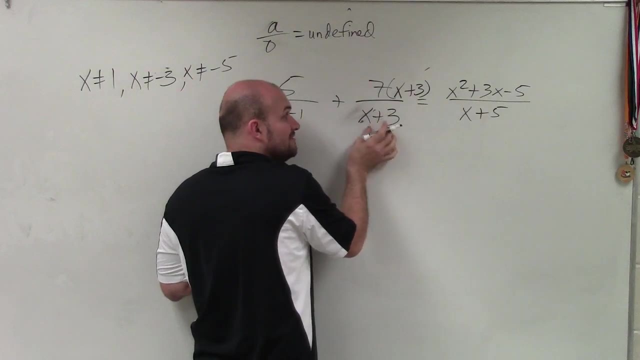 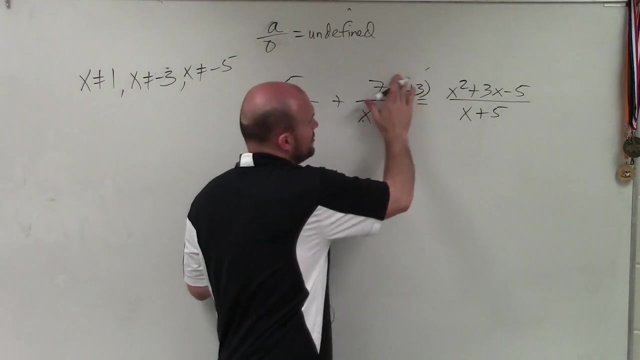 actually factor out. for instance, if I had something like this in my equation, we can factor out the x plus x plus 3, correct? Therefore, even though it's still a restriction, my value x can still not equal negative 3.. However, it's going to produce a hole, not actually an asymptote.